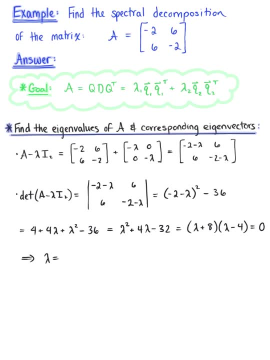 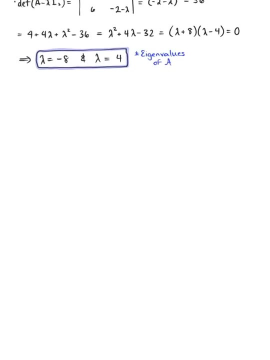 which leaves us with the eigenvalues: lambda is equal to negative 8 and lambda is equal to 4.. So now that we have these eigenvalues of our given matrix A, we need to find their corresponding eigenspaces to identify the eigenvector for each eigenvalue. So case number 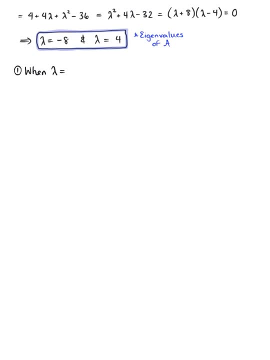 1, we need to consider when lambda is equal to negative 8.. Now we are looking for the null space of the matrix A plus 8 times the eigenvalue of the matrix A, So we need to find the eigenvector. 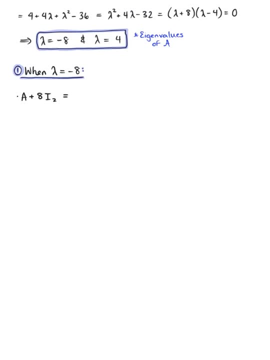 for each eigenvalue. So case number 1, we need to consider when lambda is equal to negative 8.. So we need to find the eigenvalue of the matrix A plus 8 times the 2 by 2 identity. So our given: 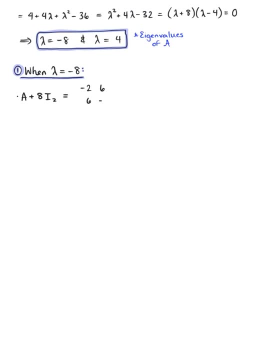 matrix A is negative. 2,, 6,, 6, negative 2, and we are adding the 2 by 2 matrix 8, 0,, 0,, 8.. Combining up these like terms, we are left with the cute 2 by 2, matrix 6,, 6,, 6, 6.. 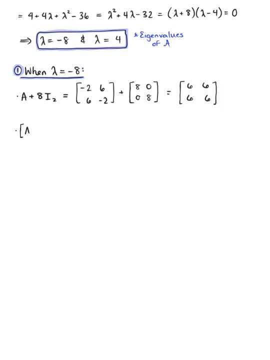 Now to find the null space, we are going to augment this matrix with the zero vector. So, taking the matrix we just found, we can immediately reduce both rows by multiplying each row by a factor of 1, 6, which leaves us with the 2 by 2 matrix: 1, 1,, 1, 1.. 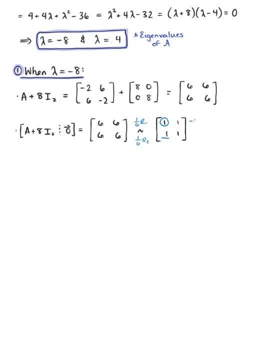 And taking our first pivot, we can use it to eliminate the entry below it. by doing minus, the first row times the second row, Which leaves us with the matrix 1, 1, 0, 0.. So this matrix is in row-reduced echelon form and it's letting us know that x sub 1 is equal to. 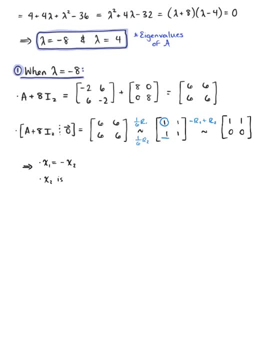 minus x sub 2, and that x sub 2 is a free variable. So we can say that the solution set vector x is the set of all vectors in R2, where x sub 1 is the set of all vectors in R2.. 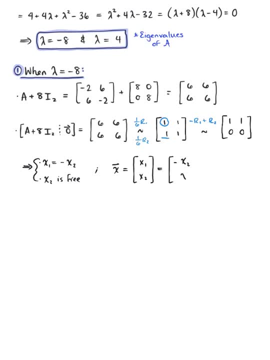 And that x sub 1 is defined as minus x sub 2, and x sub 2 is just itself because it's a free variable. So pulling out that common scalar, x sub 2,, we have x sub 2 multiplied by the vector negative 1, 1.. 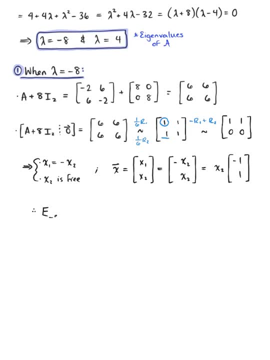 So we can conclude that the eigenspace that corresponds to the eigenvalue lambda equals negative 8- is defined by the set spanned by the vector negative 1, 1.. Beautiful, And very similarly we need to do the same thing for our second eigenvalue. 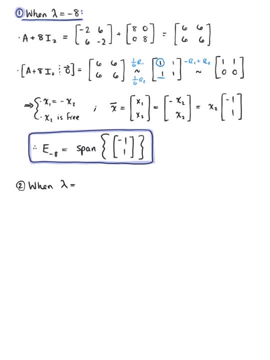 So we need to consider when lambda is equal to 4. And we need to find the null space of the matrix A minus 4 times the 2 by 2 identity. So our given matrix A is negative 2,, 6, 6, negative 2.. So we need to find the null space of the matrix A minus 4 times the 2 by 2 identity. So we need to find the null space of the matrix A minus 4 times the 2 by 2 identity. So we need to find the null space of the matrix A minus 4 times the 2 by 2 identity. 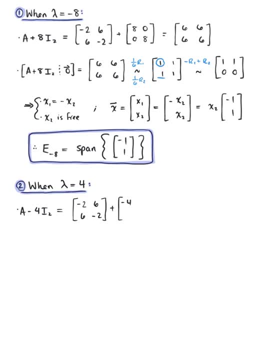 And we are adding the 2 by 2 matrix negative 4, 0, 0, negative 4.. Combining up these like terms, we are left with the 2 by 2 matrix negative 6, 6, 6, negative 6.. 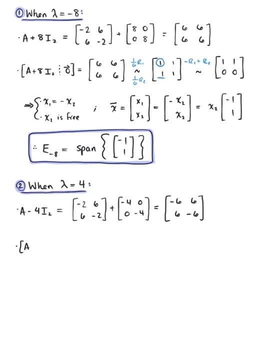 Now to find the null space again, we are going to augment this matrix with the 0 vector and row reduce to row reduced echelon 4.. So taking that 2 by 2 matrix we just found, we can again immediately simplify. 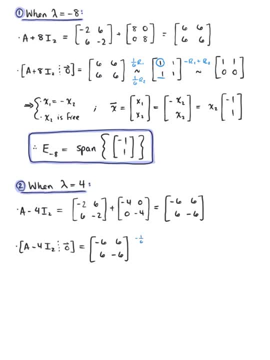 by multiplying each row by a scalar multiple of 1, 6.. So, excuse me, negative 1, 6.. Which leaves us with the matrix 1, negative 1, negative 1, 1.. And using our first pivot to eliminate the entry below it, we can do this by simply adding. 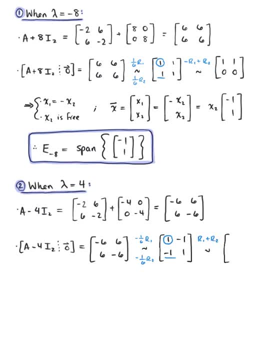 the first pivot to the next entry below it. So we can do this by simply adding the first pivot to the next entry below it. So we can do this by simply adding the first row to the second row, Which leaves us with the row equivalent matrix 1, negative: 1, 0, 0.. 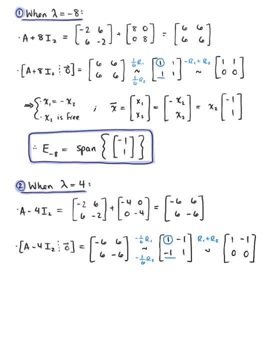 Which is in row reduced echelon form. Woohoo, And this matrix, reduced matrix- is letting us know that x sub 1 is equal to positive x sub 2. And that x sub 2 is a free variable. So we can say that the solution set is the set of all vectors x. 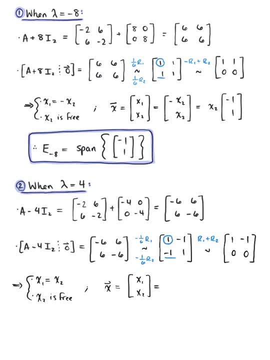 in R2, where x sub 1 is equal to x sub 2, and x sub 2 is itself because it's a free variable, And factoring out that common scalar, multiple x sub 2, we're left with the vector 1, 1.. 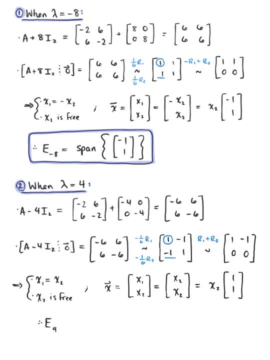 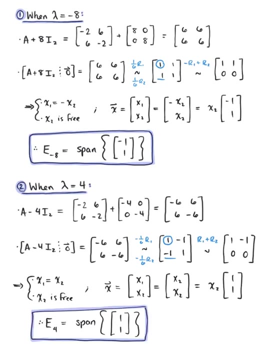 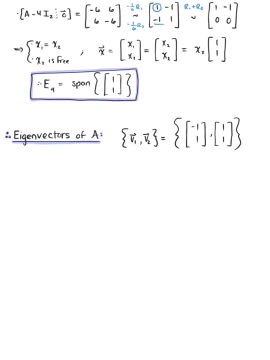 So therefore, the eigenspace corresponding to the eigenvalue lambda equals 4 is equal to the span of the vector 1, 1.. So we can do this by simply adding the first pivot to the next entry below it. Now, with these two eigenspaces, we can conclude that the eigenvectors of matrix A are the vectors v sub 1 and v sub 2.. 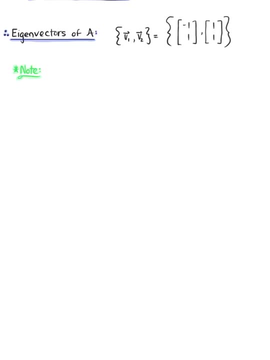 Now, observing these eigenvectors, we can see that they're orthogonal. We know that the dot product of these two eigenvectors is equal to 0. But unfortunately they're not unit vectors. So in order to be able to find the orthogonal matrix Q, we need to normalize the eigenvectors. 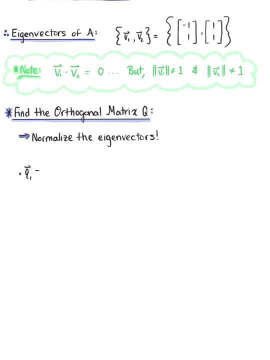 So we can go ahead and let column vector Q sub 1 be defined by normalizing eigenvector v sub 1.. So eigenvector v sub 1 has the components negative 1, 1, and finding its length. 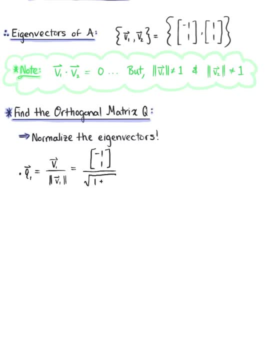 we have a vector v sub 1.. So we have the square root of negative 1 squared is 1, plus 1 squared is 1.. So we have the scalar multiple 1 by the square root of 2, multiplied by the eigenvector with components negative 1, 1.. 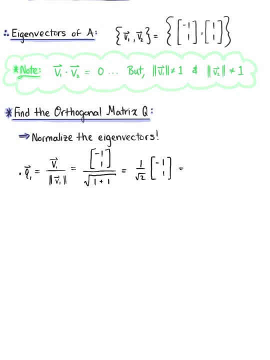 And distributing that scalar multiple through, we have the vector with components minus 1 by the square root of 2, 1 by the square root of 2.. And very similarly for column vector Q sub 2, we can define this: 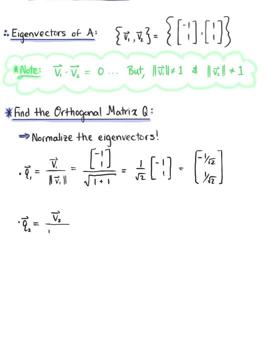 So we can define this column vector by normalizing eigenvector v sub 2.. So vector v sub 2 has the components 1,, 1, and fortunately the length of this vector is the same square root of 2.. 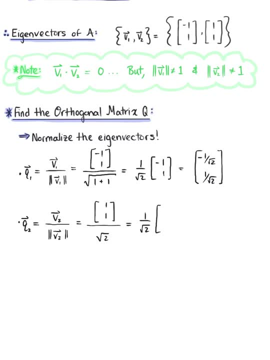 So we have that scalar multiple: 1 by the square root of 2, multiplied by the vector with components 1, 1, which leaves us with the vector with components 1 by the square root of 2, 1 by the square root of 2.. 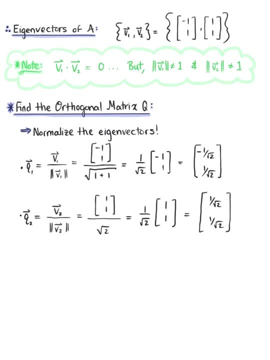 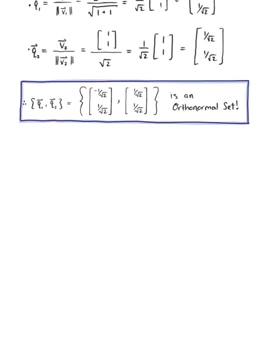 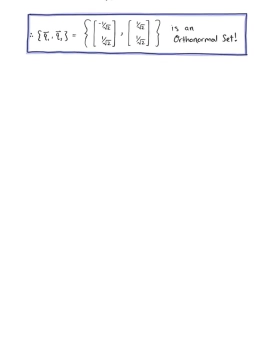 So we can conclude now that the set Q sub 1, Q sub 2, defined by these two vectors, is an orthonormal set. Now the last thing that we need to do before we can officially write this spectral decomposition is to compute the product of each vector Q sub i with the transpose of vector Q sub i. 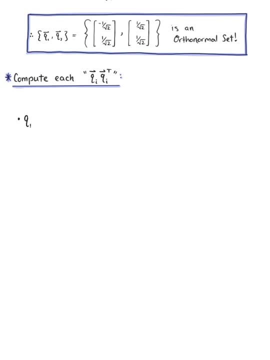 So our first vector is the transpose of vector Q sub i And the second is the transpose of vector Q sub x. The first product is the vector Q sub 1 multiplied by the transpose of vector Q sub 1.. So we can take the vector Q sub 1 that we just found above and multiply this by the transpose. 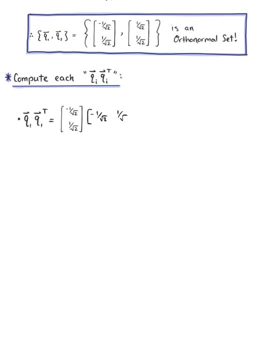 So we have the vector negative: 1 by the square root of 2,, 1 by the square root of 2.. Now by the row column rule of matrix multiplication, we've added the travelled product. So I just want to let 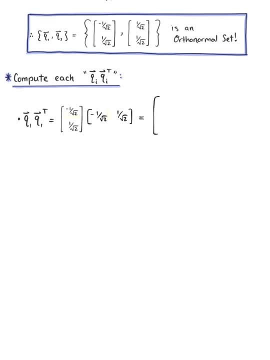 multiplication: we have the first row by the first column, which leaves us with 1 half. We have the first row by the second column, which leaves us with negative 1 half. Second row by the first column leaves us with minus 1 half, and the second row by the second. 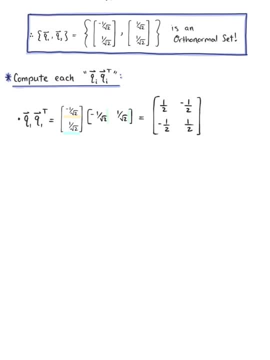 column leaves us with positive 1 half. We also need to compute the product vector q sub 2, multiplied by the transpose of vector q sub 2.. And again, taking the vector q sub 2 that we found above, we now want to multiply this. 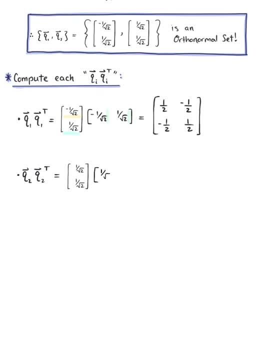 vector by its transpose: 1 by the square root of 2, 1 by the square root of 2.. And again, applying the row-column rule for matrix multiplication, we have the first row by the first column, Which gives us 1 half. 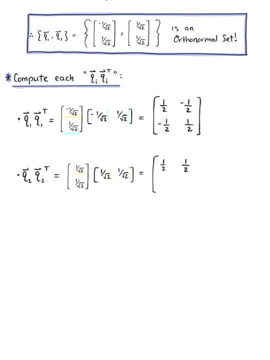 The first row by the second column gives us 1 half, And we have the second row times the first column, which leaves us with 1 half, And the second row by the second column, which also leaves us with 1 half. Beautiful.